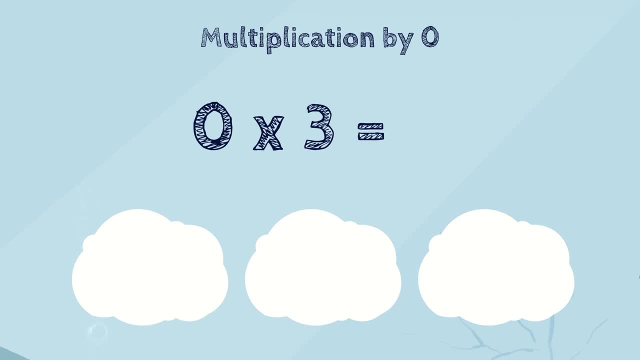 What will it be in total Nothing, Yes, it's a total Nothing. Yes, a total Yes. But what are the groups of zero? Nothing, Das right. The three groups of zero in total Zero. Yes, Yes, sure, It will be nothing or zero. And what if we multiply zero by five? 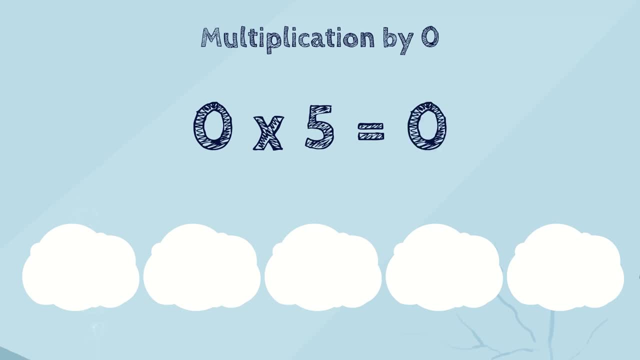 It's still nothing. Yes, No matter how many times we add nothing, the answer is always nothing. So if zero is multiplied by any number, the answer is always zero. We also know that we can move numbers around and it doesn't change the answer, So it doesn't matter where your zero is placed. 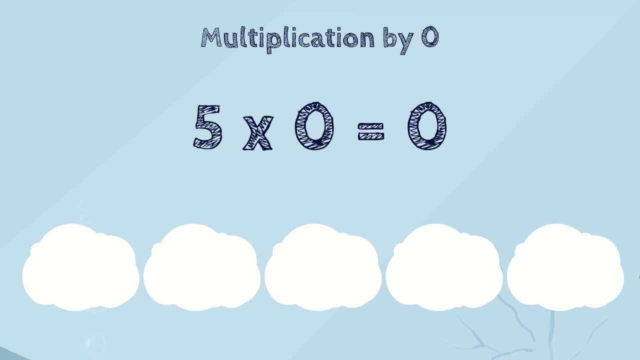 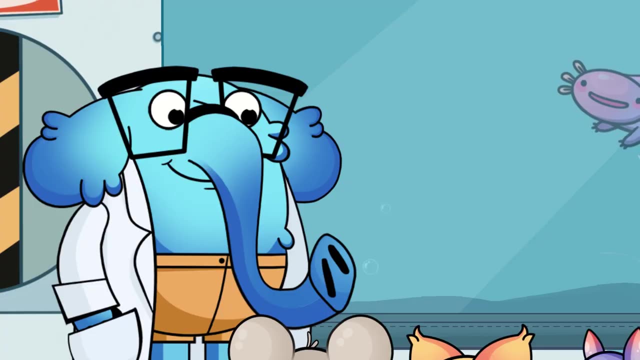 If you just see the number zero as one of the numbers multiplied in your multiplication problem, then your answer is zero. So, kids, what is a million times zero? Zero, That's right. Let's repeat the tricks that we've learned today. 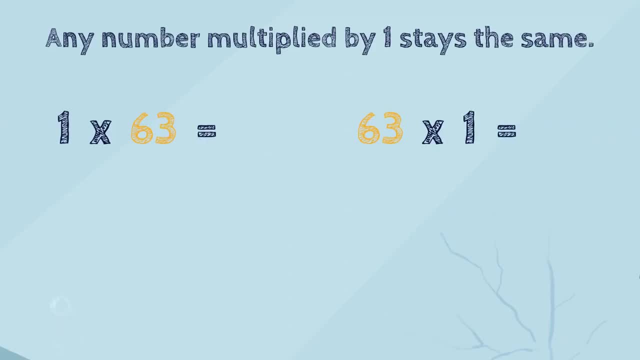 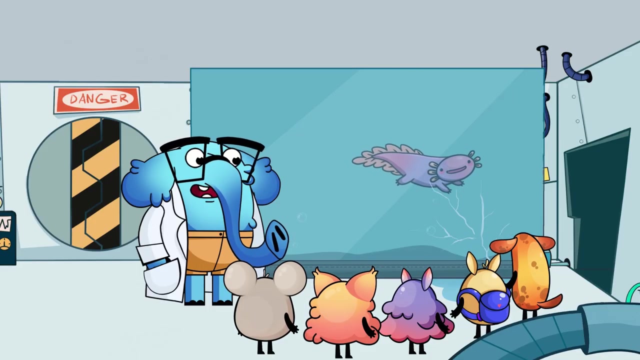 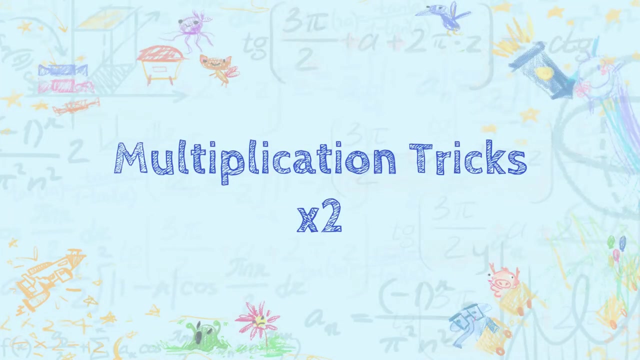 The first trick is that any number multiplied by one stays the same. The second trick is that any number multiplied by zero makes zero. I think that's enough for today. Next time I will show you some more tricks. Hello kids, Hello professor. 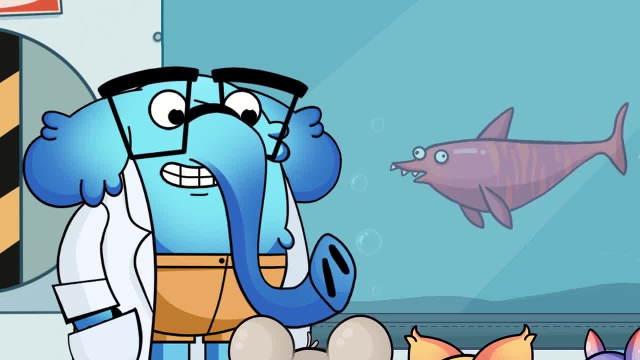 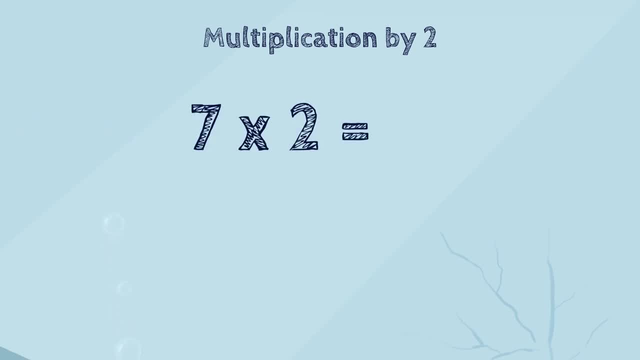 Kids. today we'll discuss multiplication by two. Let's look at the example Seven times two. What does this mean? It means we have two groups of seven items, and so we need to add seven two times. That will be seven plus seven. 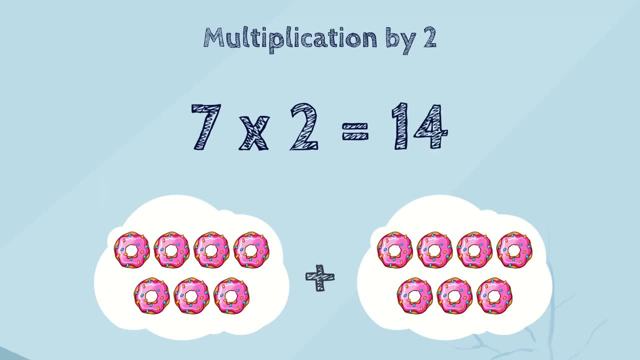 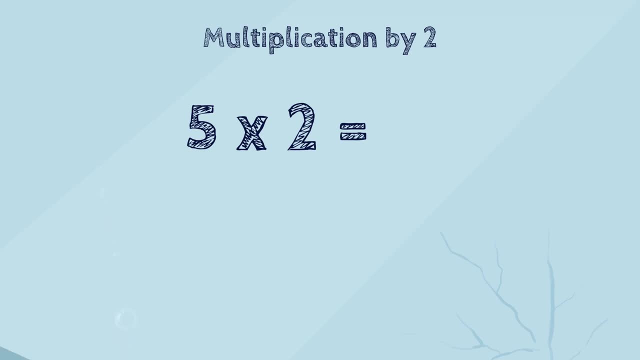 So what will? What will the answer be Fourteen, Yes, that's true. Now let's look at five times two. How would you solve this problem? Five plus five, Yes, and that is Ten. Great, You've understood the idea. 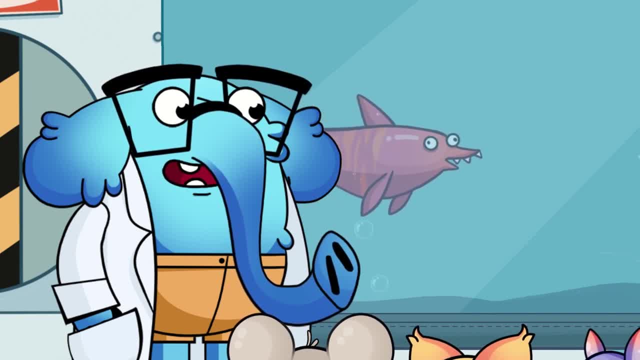 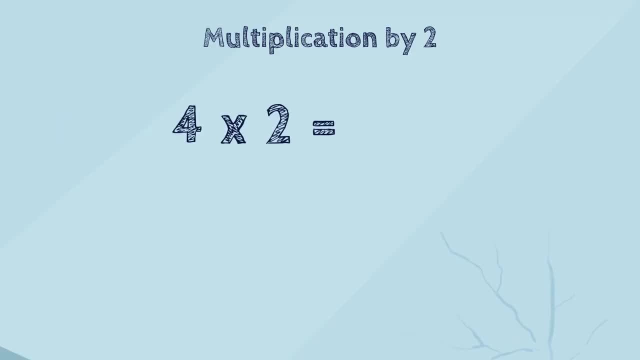 Multiplication by two means that you just need to add the number twice, So you can always get the answer easily. Four by two is the same as four plus four. Eight by two is the same as eight plus eight. Eleven by two is the same as eleven plus eleven. 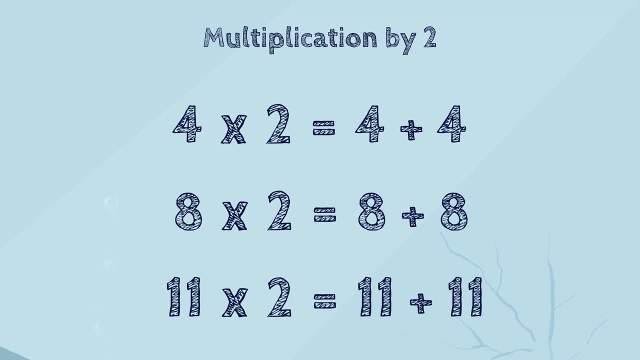 We also know that the order of numbers in multiplication does not change the answer, So it doesn't matter where two is placed. It can be first or second. We can still use this trick. Let's think about how to solve twenty times two. 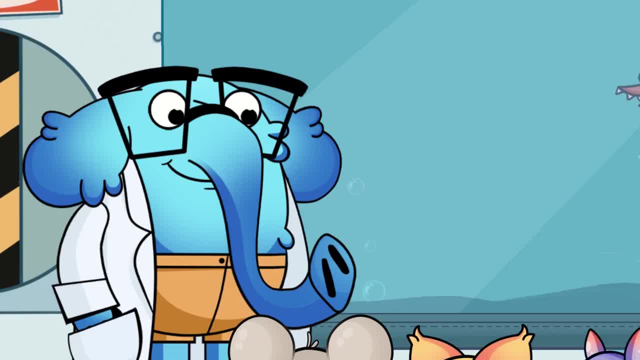 Add twenty twice And that will be Forty, You're right. So let's remember this simple trick: To multiply by two, you just need to double the number. That's it for today. Next time we'll discuss some tricks using multiplication. 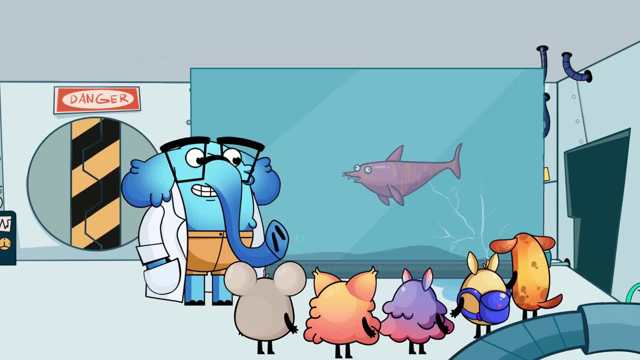 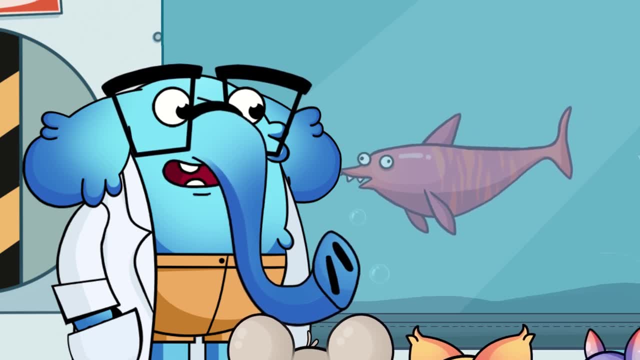 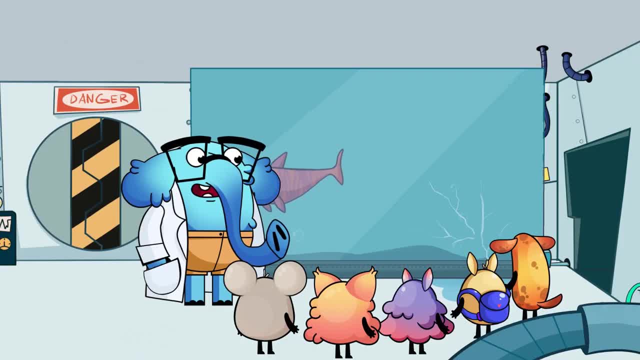 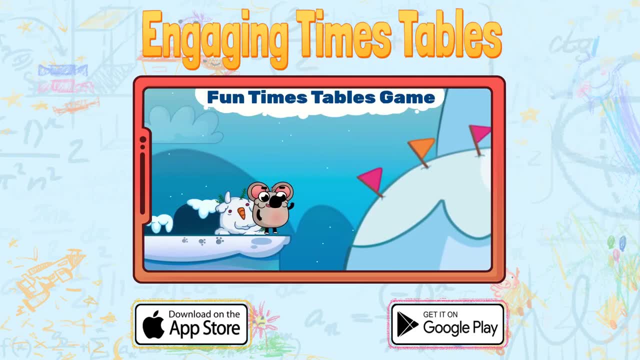 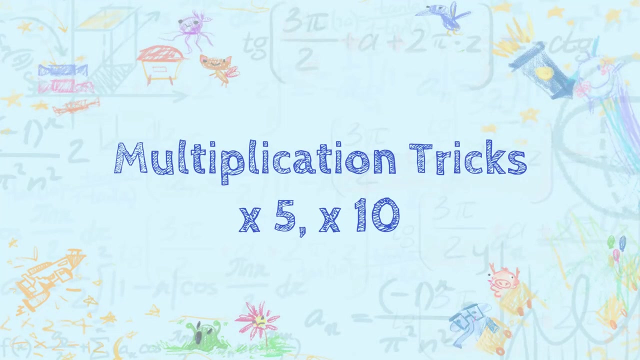 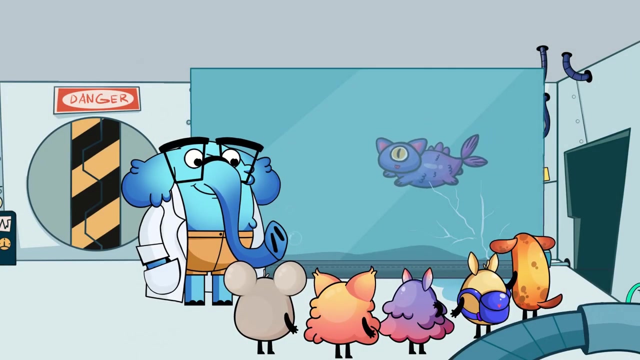 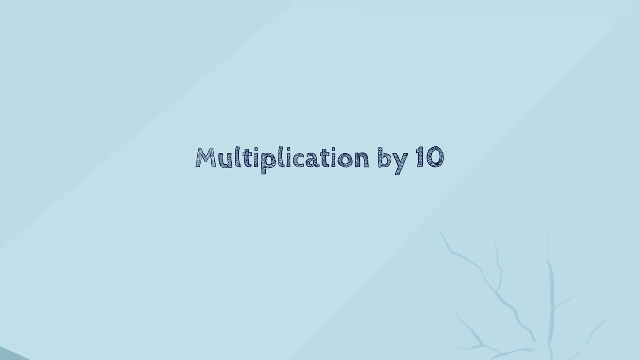 Bye-bye, Bye-bye, Bye-bye, Bye-bye, Bye-bye, Bye-bye, Bye-bye, Hello kids, Good morning, Professor five. Let's start with multiplication by ten and look at some examples. We know that one times ten 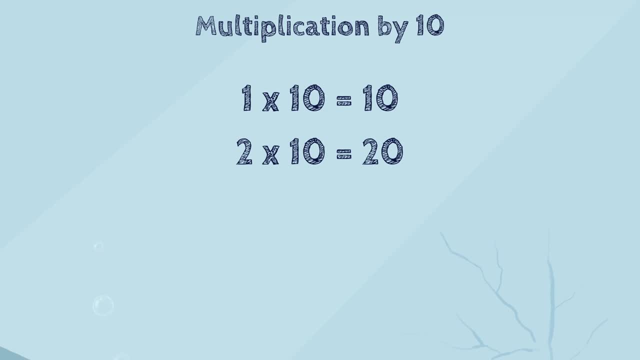 is ten, two times ten is twenty, three times ten is thirty, four times ten is forty, and five times ten is fifty. Have you noticed something interesting, kids? It looks like you just add a zero to the number that you multiply by ten. Yes, absolutely, You've found the trick and I can say that it works. 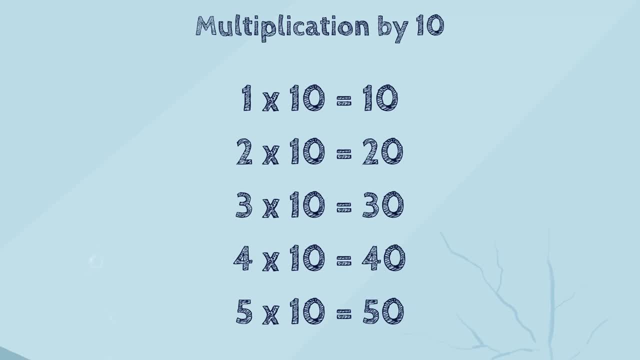 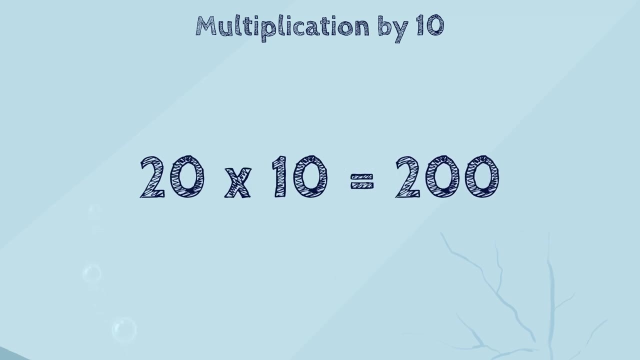 for any number that you multiply by ten, You just need to add zero to it. So let's try: twenty times twenty, What do you think? the answer is Two hundred. Yes, and we all also know that. the order of the numbers 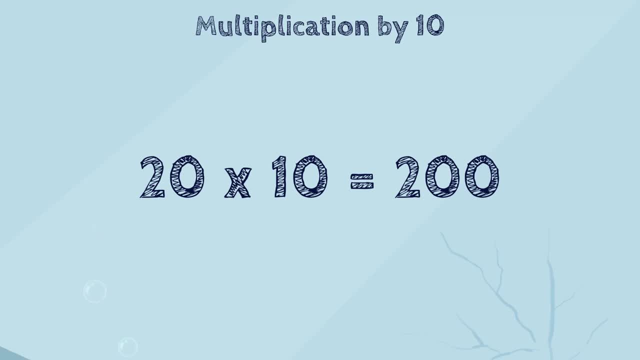 doesn't matter in multiplication, so this trick can still be used if ten is the first number too. Ten times twenty equals two hundred, and twenty times ten equals two hundred. Let's try to solve another problem: What is ten times twenty? 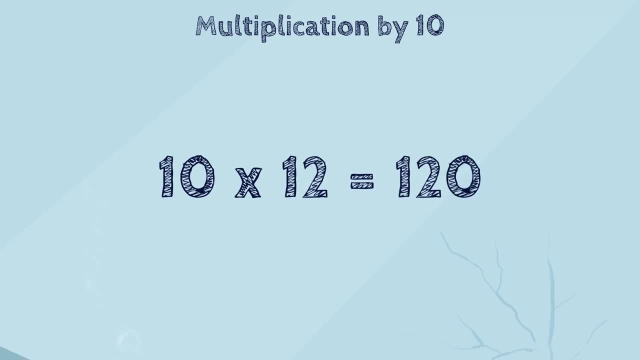 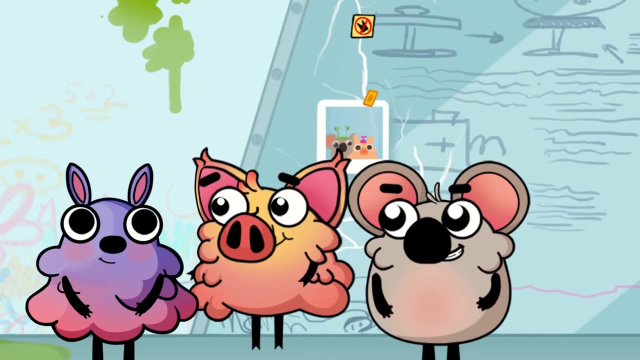 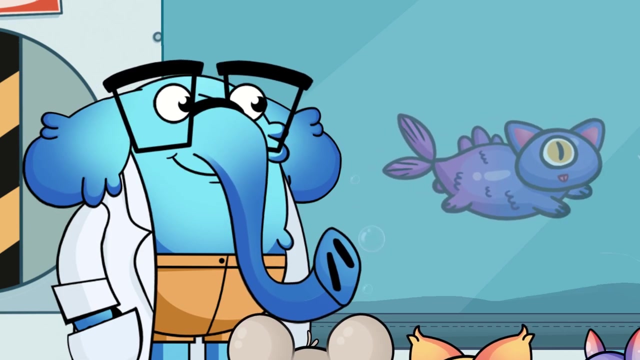 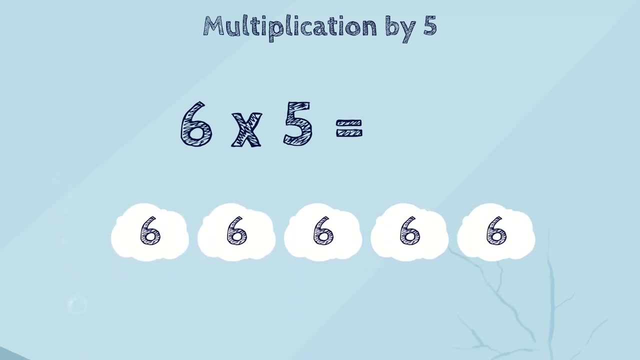 Twelve, One hundred and twenty. Yes, that's it. I think you understand the trick. Yes, this is really helpful. Okay, now let's look at multiplication by five. What is six times five? It means that we need to add six five times, but we've just learned the. 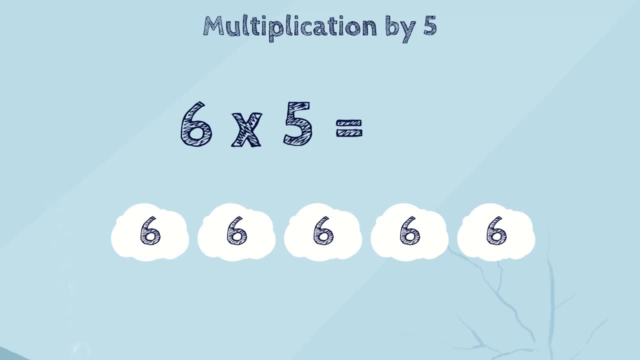 trick to multiplication by ten, so you can see that we need to add six five times. but we've just learned the trick to multiplication by ten, so we can easily find the answer to adding six, ten times. You know that sixty. Now what is five in comparison to ten? 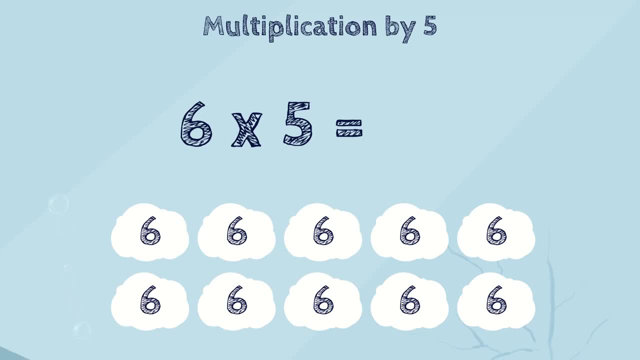 Is five, half of ten. Yes, you got that. Five is half of ten. So to multiply any number by five, you could multiply it by ten and then take half of that answer. Let's return to our example. The problem was: what is six times five? First we'll multiply six times ten, That's sixty. 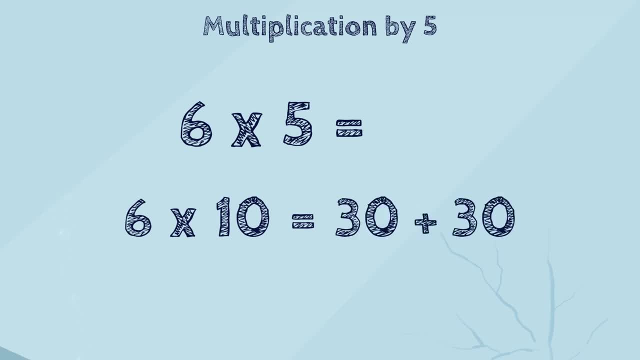 Then we'll take half of sixty, That's thirty. So six times five is thirty. Let's try one more problem: Twelve times five, We can easily figure out that twelve times ten is one hundred and twenty. And then what is six times five? That's sixty. So six times five is thirty. And then 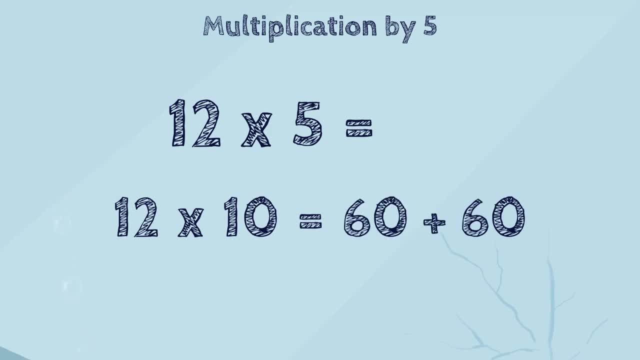 is half of 120, it's 60. yes, that's right. so 12 times 5 is 60. as always, we remember that the order of the numbers doesn't change the answer in multiplication, so it doesn't matter if 5 is the first or the second number. this: 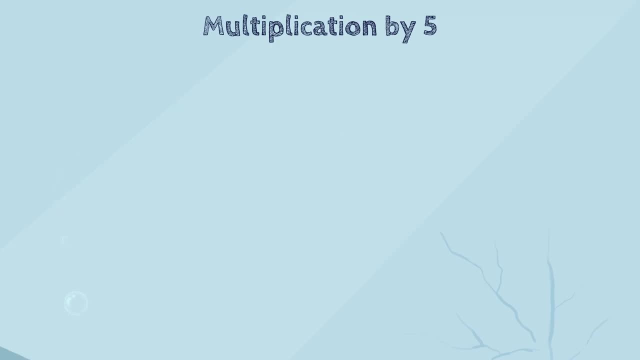 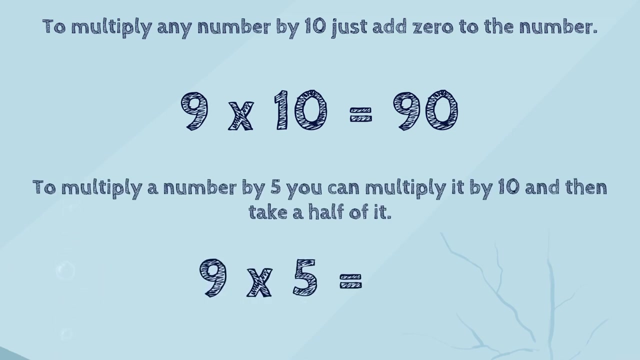 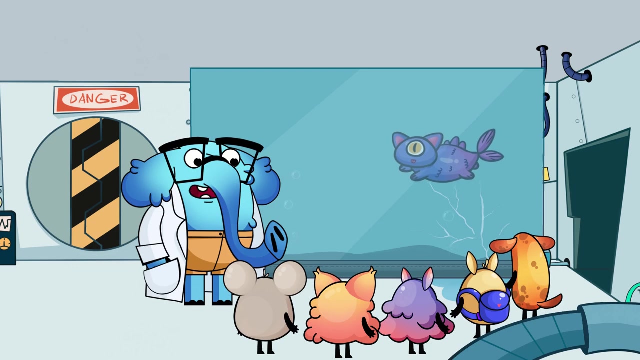 trick can still be used. let's repeat the tricks we've learned. to multiply any number by 10, just add 0 to the number. to multiply a number by 5, you can multiply it by 10 and then take half of it. that's it for today. next time we'll learn some new tricks. 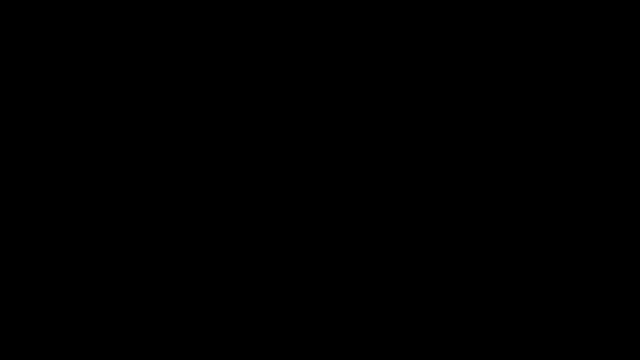 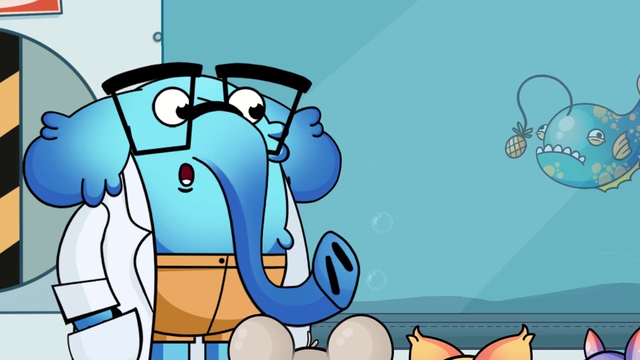 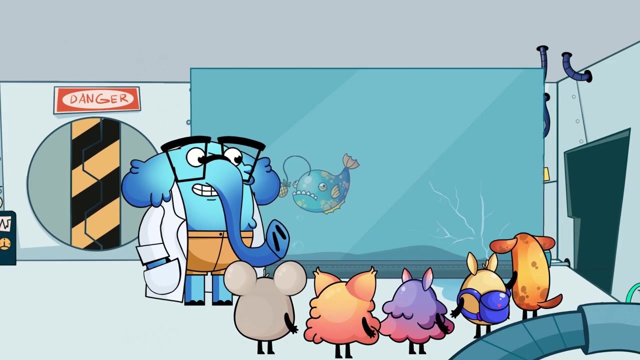 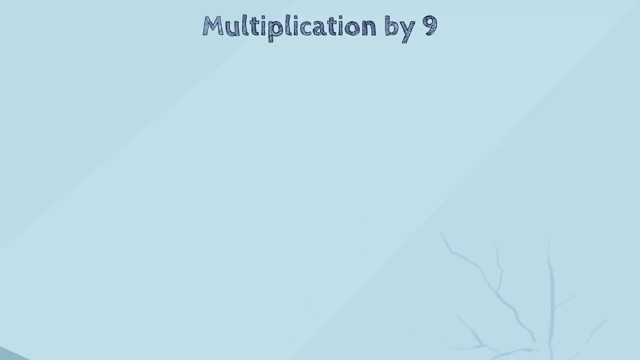 you. hello kids, hi. today we'll continue to discover multiplication tricks, and we'll look at multiplication tricks by 9. I'll show you two different tricks. either can be used to find the answer in multiplication, so let's start with the first one. what is 7 x 9? 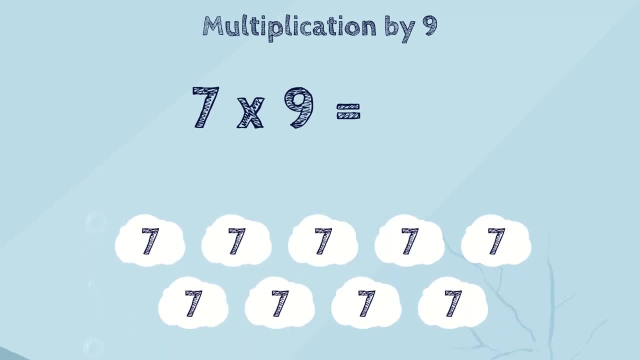 it can be seen as nine groups of seven items. so to get the answer in multiplication we need to add 7- 9 times. it doesn't look that easy. oh, this isn't the whole trick yet. so to find the answer we need to add 7- 9 times, and I. 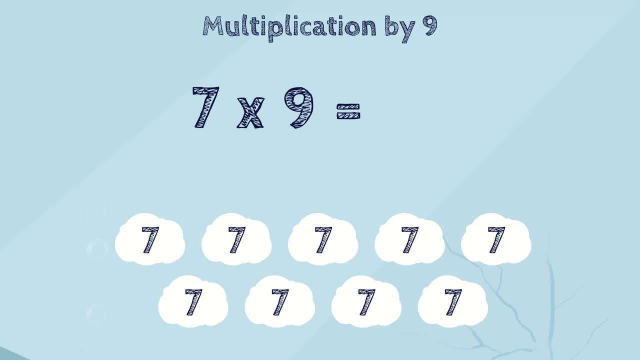 agree with you, Kelly. it really doesn't look easy. but what can we do easily? we know how to easily add 7 10 times. that'll be 7 times 10 and that's 70. so we know the answer when adding 10 sevens. but we need only nine in this problem. 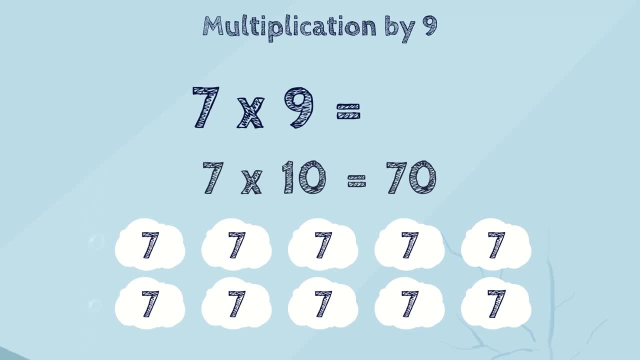 what can we do? maybe subtract 17? yes, you're right, if you know the answer- of adding 10 7s, but you need only 9 7s. you can subtract 1, 7 from the answer, So it will be 70 minus 7,. 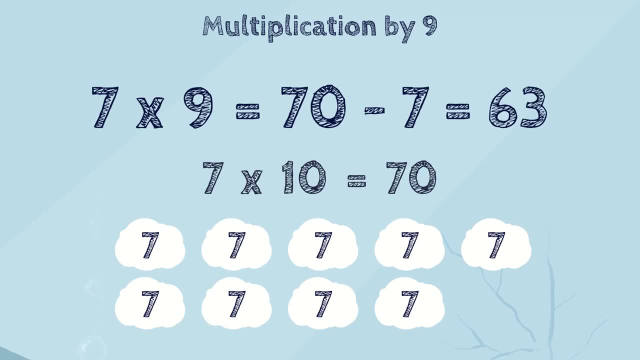 and that's 63. So 7 times 9 is 63.. Let's summarize this trick: To multiply a number by 9, you can multiply it by 10 and then subtract the number that you are multiplying by 9.. 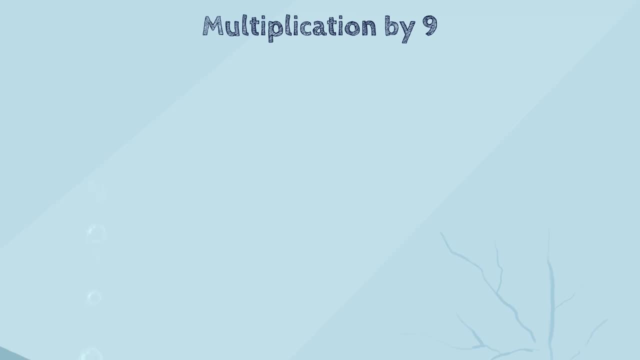 Let's try several more examples. What is 5 multiplied by 9?? 5 times 9 is 5 times 10 minus 5.. 5 times 10 is 50.. 50 minus 5 is 45.. So 5 multiplied by 9 is 45.. 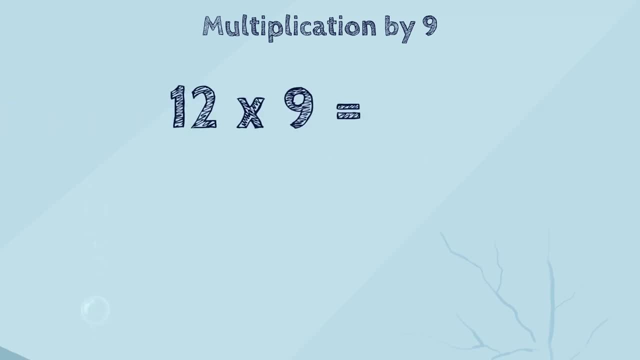 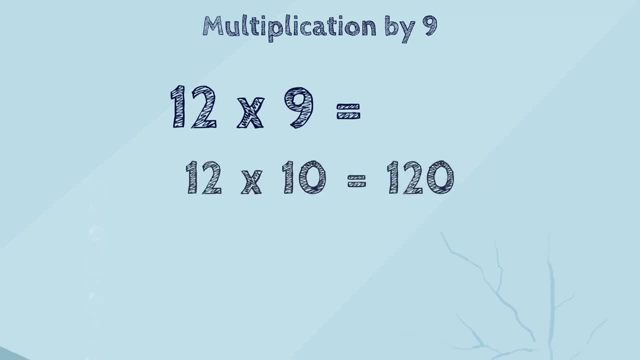 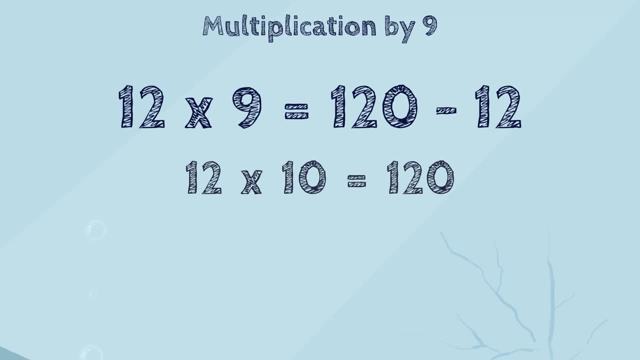 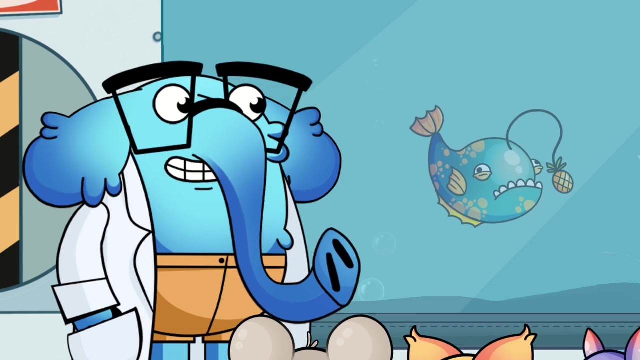 Hmm, 120 minus 12 is 108.. So that means 12 times 9 is 108.. Yes, that's right, Kelly. Great job. Now let's look at another way to multiply by 9.. I call it the magic hands trick. To use this trick, put your hands straight out in front of you. 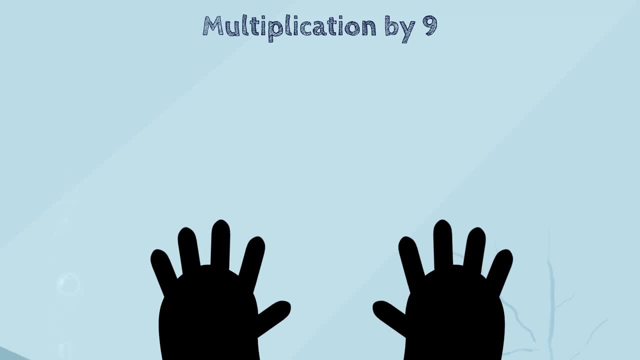 Don't bend your fingers. Let's count your fingers from 1 through 10, starting from the left hand: 1,, 2,, 3,, 4,, 5,, and then 6,, 7,, 8,, 9,, 10 on the right hand. 1,, 2,, 3,, 4,, 5, and then 6,, 7,, 8,, 9,, 10 on the right hand. 1,, 2,, 3,, 4,, 5, and then 6,, 7,, 8,, 10 on the left hand. 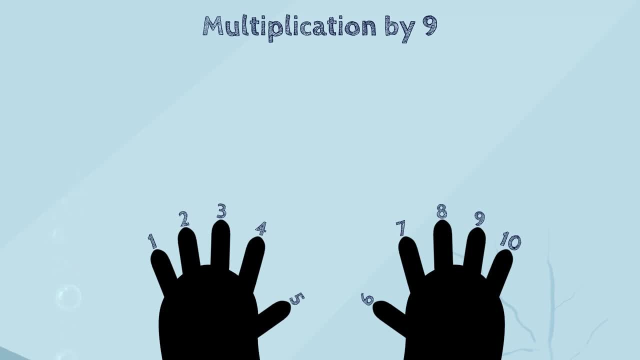 1,, 2,, 3,, 4,, 5,, and then 6,, 7,, 8,, 10 on the right hand. Now let's say that you would like to multiply 3 by 9.. To do this problem, you need to fold down the finger of the number you want to multiply by 9.. 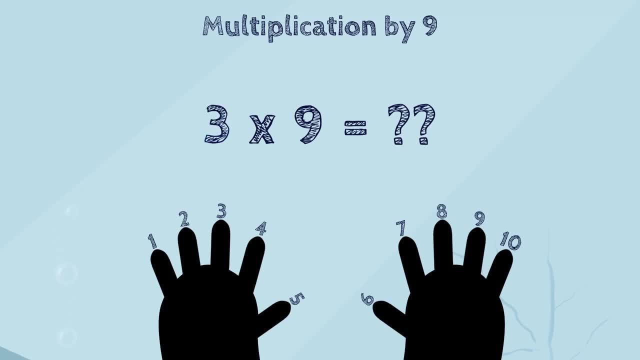 In this case we need to fold down the third finger because we are multiplying 3 by 9.. So count the numbers on the left hand until you get to 3.. Start on the left side of the hand: 1,, 2,, 3.. Fold that finger down. 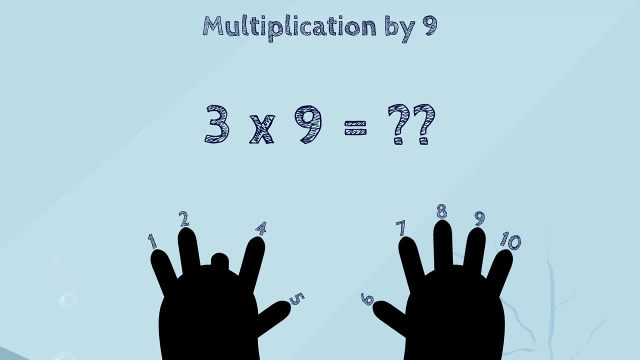 Now let's count the number of fingers to the left of the folded finger. That will be the first digit in the answer. In this case we have two fingers to the left of the folded finger, So we put 2 in the tens place for the answer. 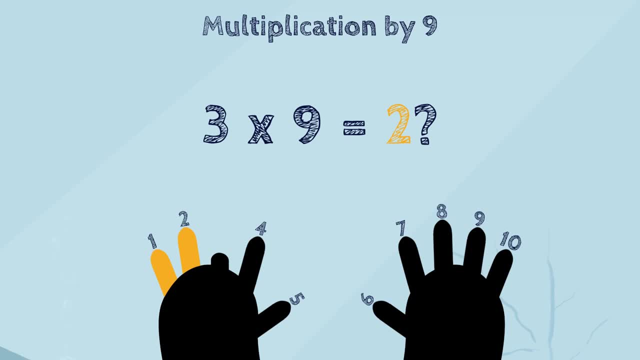 Now let's count the number of fingers to the right of the folded finger. That will be the second digit in the answer. There are 7 fingers to the right, 2 fingers on the left hand and a whole hand of fingers on the right. 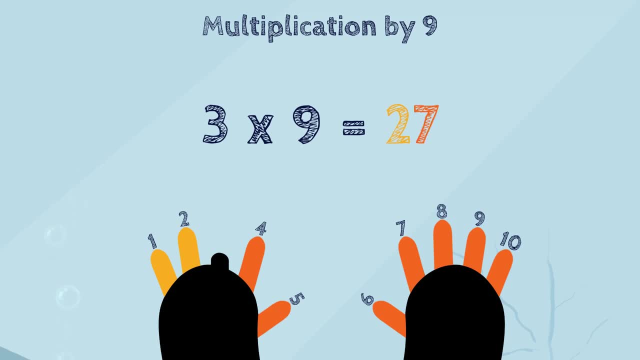 So we put the 7 in the ones spot. As a result, we have found that we know what 9 times 3 is: It's 27.. Now let's multiply 7 by 9.. To do this problem, you need to fold down the finger of the number you want to multiply by 9.. 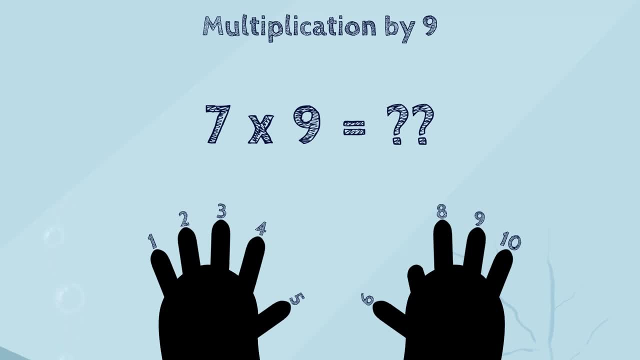 To do this, we'll fold down the 7th finger. So now we have 6 unfolded fingers to the left of the folded finger and 3 unfolded fingers to the right. So the answer to 7 times 9 is 63.. 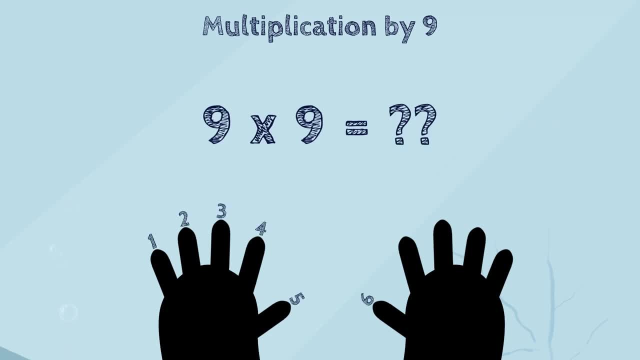 Let's try another example: 9 multiplied by 9.. We fold down the 9th finger and count the fingers to the left and then to the right of the folded finger. It will be 8 fingers to the left and 1 finger to the right. 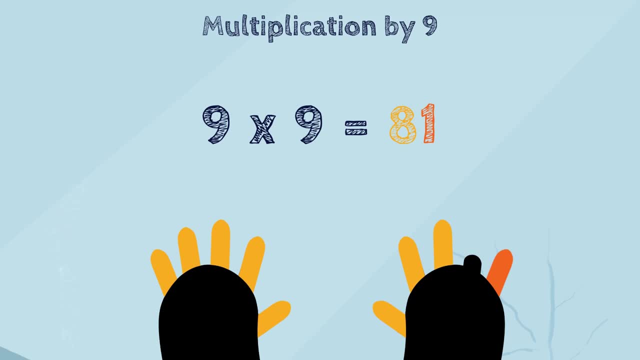 So the answer is 81.. Please remember that this trick can only be used to multiply numbers up to 10 times 9.. It can't be used to find the answer to bigger numbers like 11 times 9,, 12 times 9, and so on. 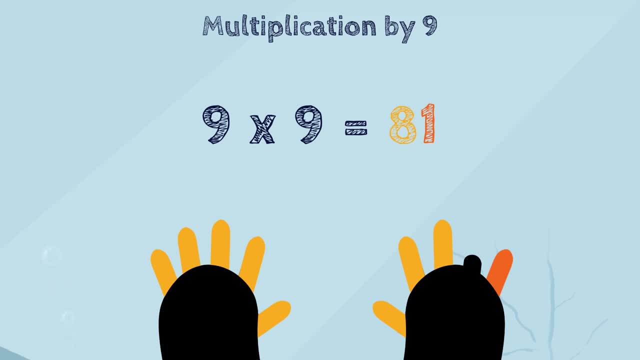 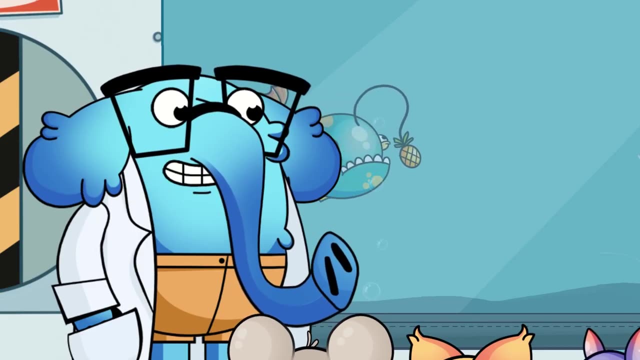 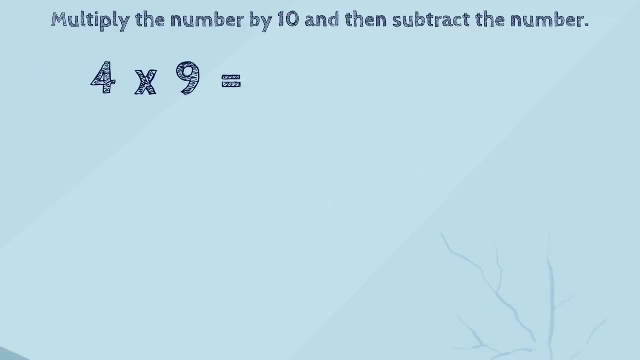 If the number you are multiplying the 9 by is bigger than 10, you can use the first trick that I showed you- let's repeat what we've learned today- to multiply a number by 9. you can use two different tricks. you can multiply the number by 10 and then subtract the number one time, or if the